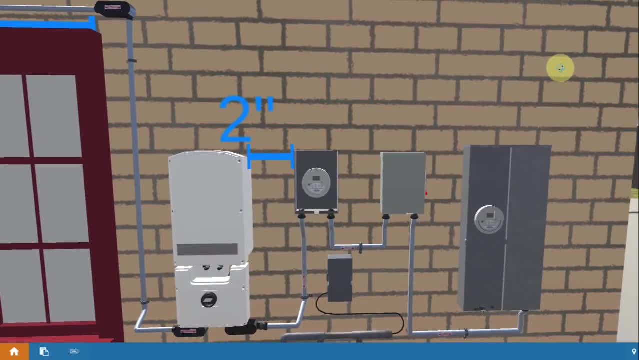 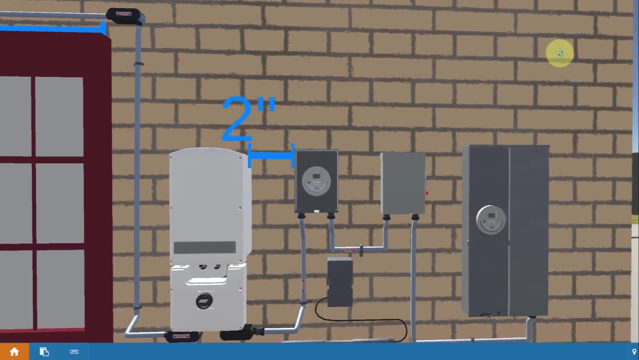 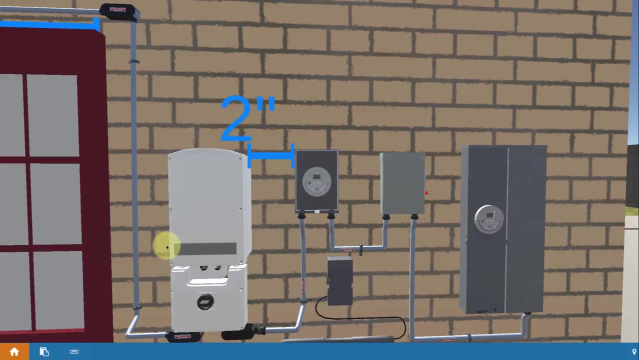 thing I want to focus on in this introduction is the electrical equipment that we're mounting on the wall. I'm going to briefly go over each one and then have separate videos describing each one further, so check those out as well. The point here is that we're being pretty generic. We've got a generic modeling, basically. 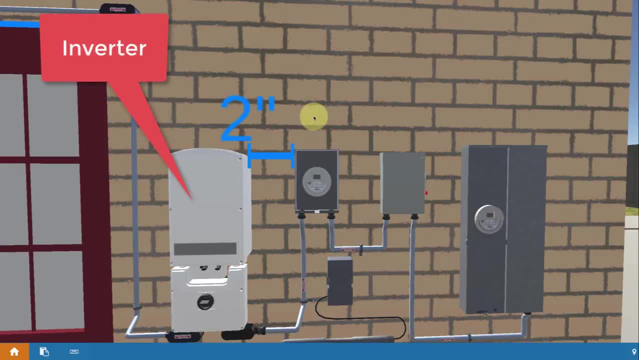 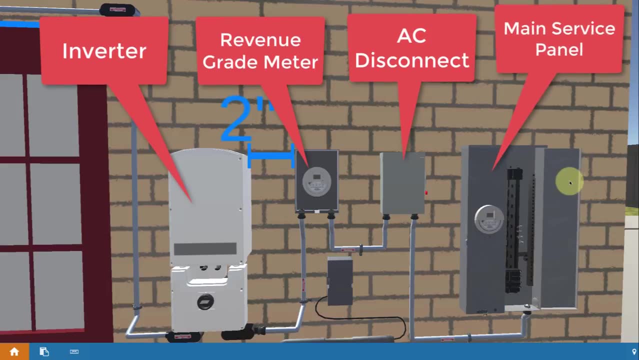 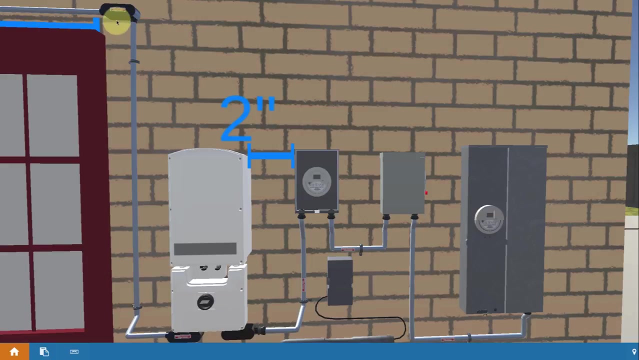 of an optimizer-based inverter. Then the power goes through a revenue-grade meter onto an AC disconnect and finally into your home main service panel. Let's go back and review these things. So the idea is that the power from the array, the DC power from the array, is going to come down and flow. 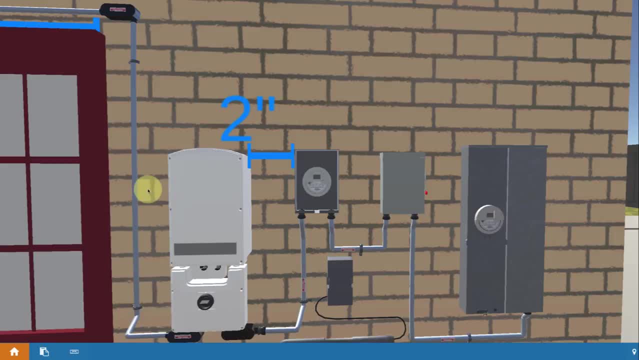 into the inverter. I'm going to describe that more in detail, But the idea is that the DC power comes into the inverter and gets converted into AC power that the house can actually use. Then the power is going to flow on to a revenue-grade meter. Now, that's an option. 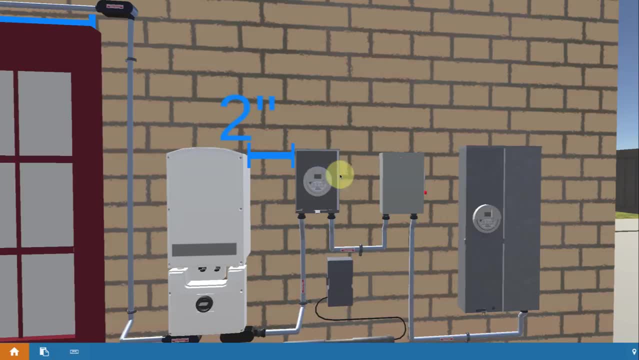 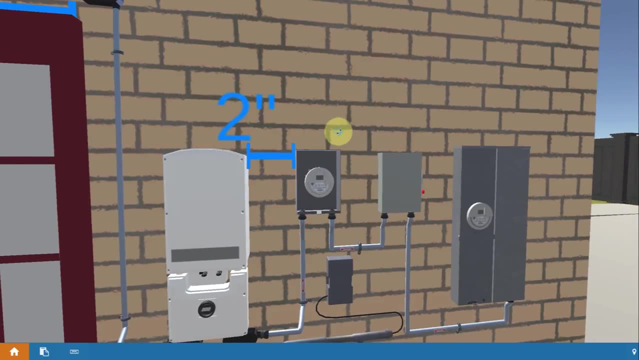 All systems don't have that. In fact, some systems now have the electronics for the revenue-grade metering built into the inverter itself, Which is very cool, But in many cases it may be a separate requirement or the inverter might not have one and you'd have to mount one. Typically, the revenue-grade meters are: 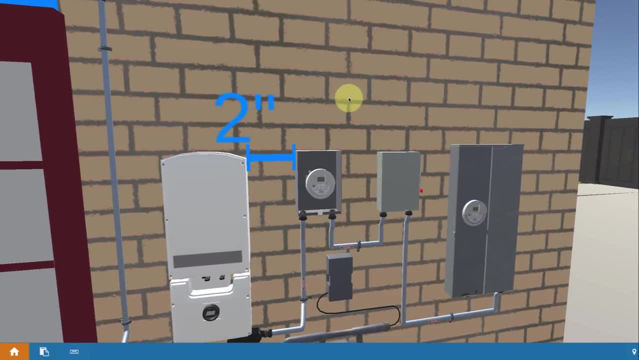 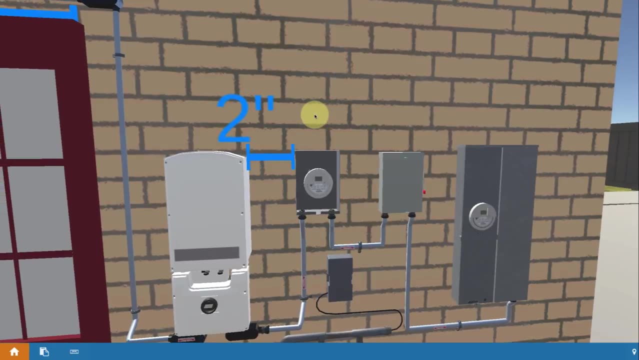 needed by the utilities to keep detailed track of the production that you've made And also if you have any sort of lease or power purchase agreement or the way that you've bought. the system requires that you monitor carefully the amount of power that's produced by the 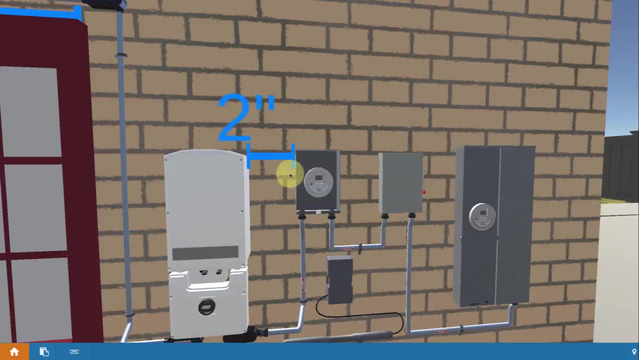 system. that's why you need the revenue-grade meter. So, again, that may be an option, but it's not always the case. If you're going to be using that option, we're going to show it installed, just for thorough-ness From. 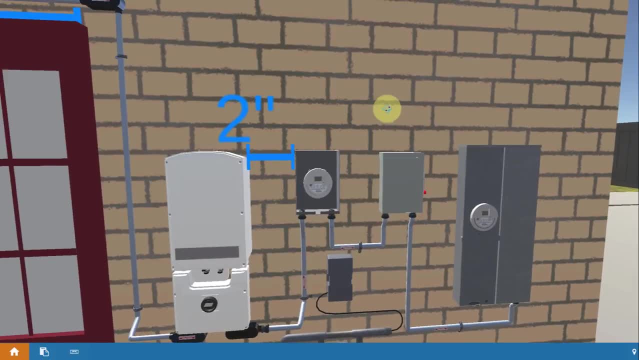 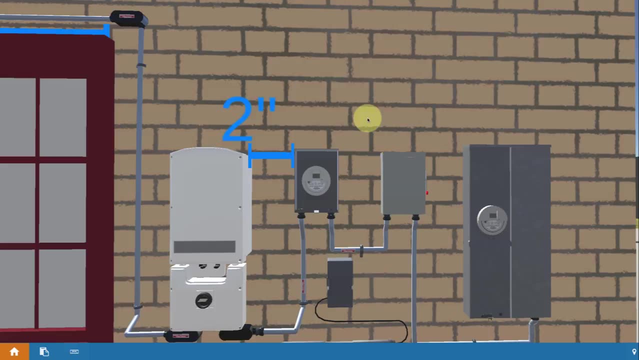 there the power comes through an AC disconnect, And there again there are some jurisdictions that now no longer require an AC disconnect switch, So you may not install one of those either, But we're going to cover it. In general, we typically see them still installed. 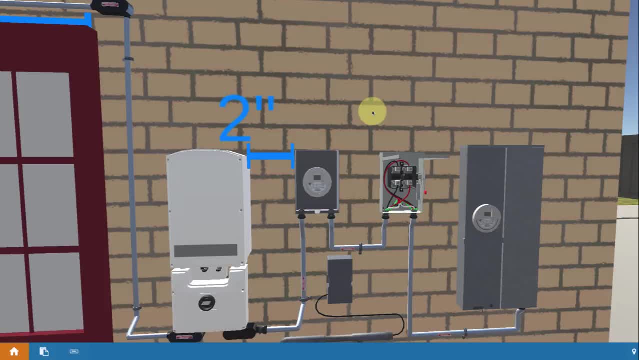 And we're actually going to show the mounting of that and eventually the wiring up of that AC disconnect. That's your main switch. You're going to see left turn on, right power off and you're going to want to tap your operating button here, The power that's connected to your电 nanometer.